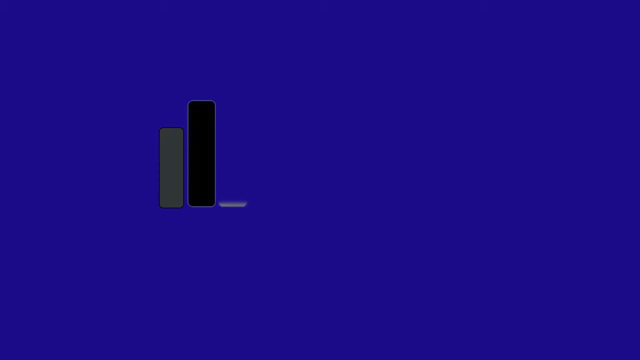 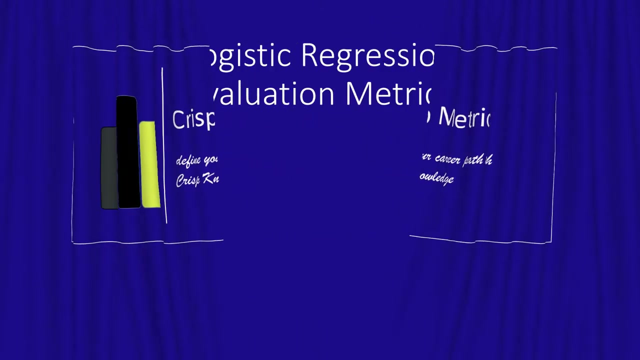 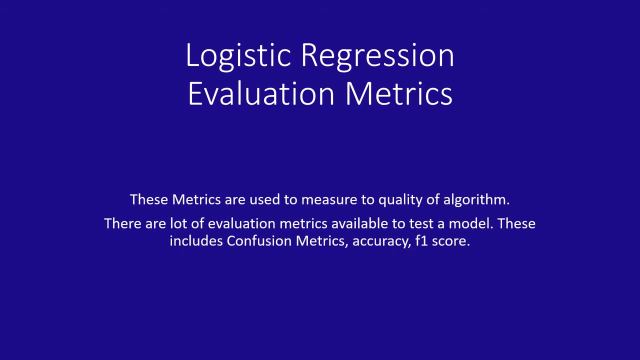 Welcome to the Crisp Metrics. In this video we will see evaluation metrics for classification algorithms. These metrics are used to measure to quality of algorithm. There are a lot of evaluation metrics available to test a model. These includes confusion metrics, accuracy, F1 score. 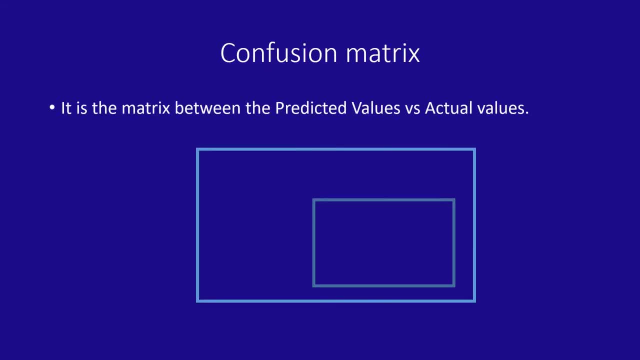 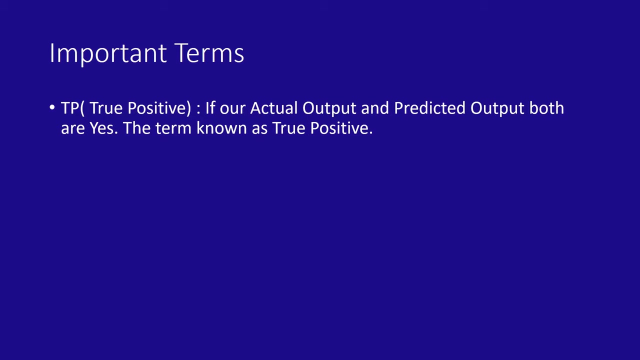 Confusion matrix. It is the matrix between the predicted values versus actual values. There are some important terms in confusion. matrix True positive if our actual output and predicted output both are yes. The term known as true positive, True negative if our actual output and predicted output both are no. 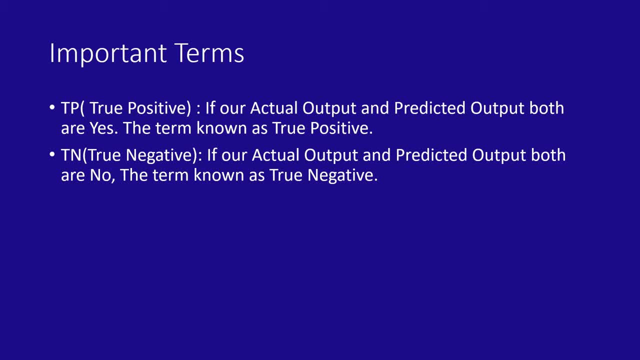 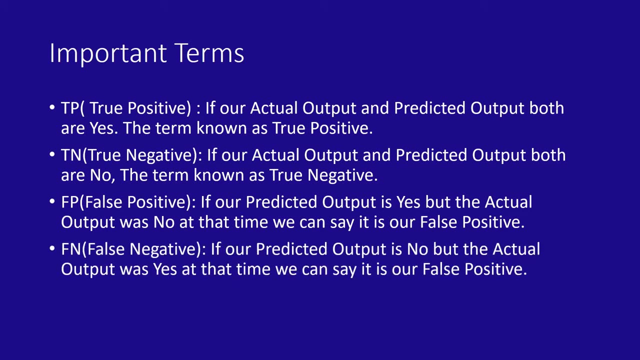 The term known as true negative- False positive. if our predicted output is yes, but the actual output was no at that time, we can say it is our false positive. False negative: if our predicted output is no, but the actual output was yes at that time, we can say it is our false positive. 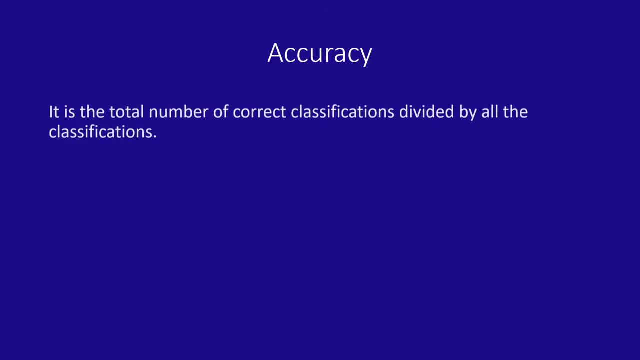 Accuracy. It is the total number of correct classifications divided by all the classifications. Correct classifications are true, positive and true- negative, because in both the cases actual and predicted values are same. Formula is true, positive, True positive plus true negative divide by all the values. 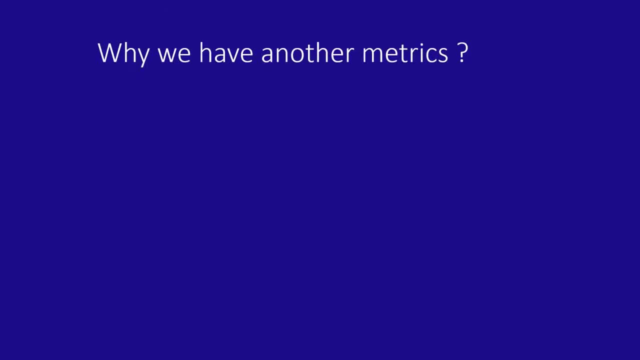 Now the question is: if we have accuracy, then why we have other metrics? Suppose, in a hospital we have 100 patients, If 60 persons have cancer and 40 persons don't have cancer. Now imagine if our confusion matrix will be like this: 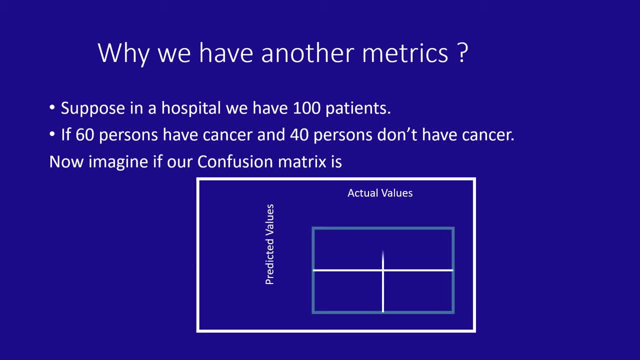 Where true positive is 30, false negative is 20, true negative is 50 and false positive is 0. Now calculate the accuracy: It will be 80%. Now, according to the matrix, it is only able to identify 30 persons with 80% accuracy. 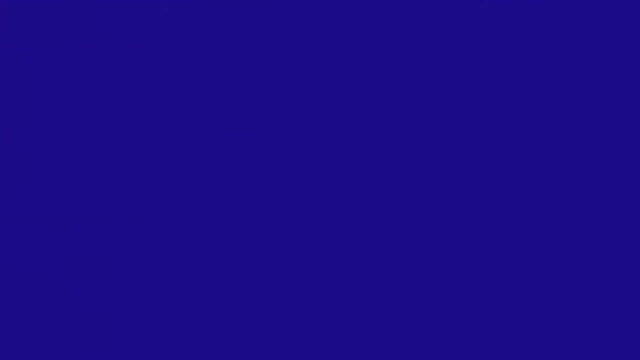 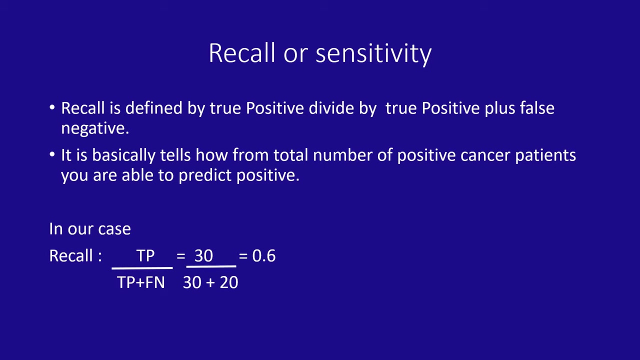 That's why we need another metrics. Next is our recall, or we can say sensitivity. Recall is defined by true positive divide, by true positive plus false negative. It is basically tells how, from total number of positive cancer patients, you are able to predict positive.